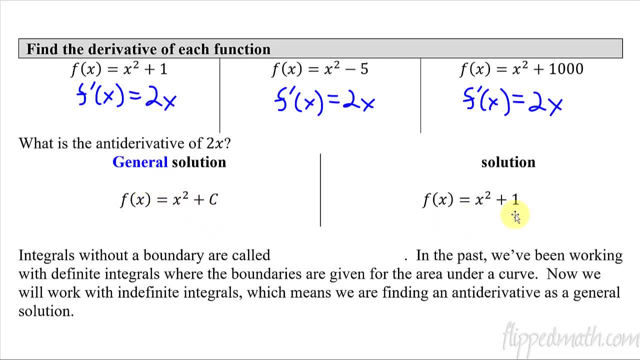 So that's what's called, again, general solution. Now, if I have a specific number here, instead of a, c, it actually is a very specific value, which in this case was the x squared plus 1, then that one's called a particular solution. It's the particular solution that fits given. 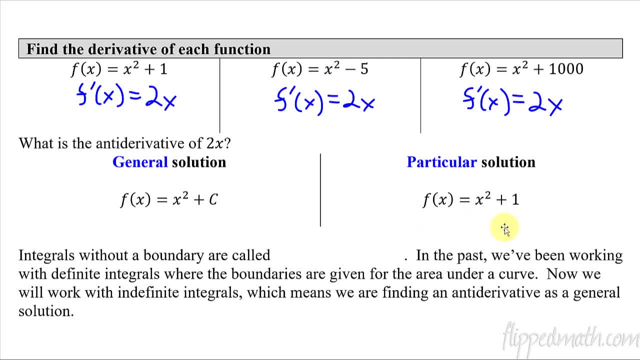 criteria, which I will show you some examples of that as we work through this lesson today. So, integrals that do not have any boundaries, these integrals without boundaries, those are called indefinite integrals as opposed to definite integrals, Definite integrals. 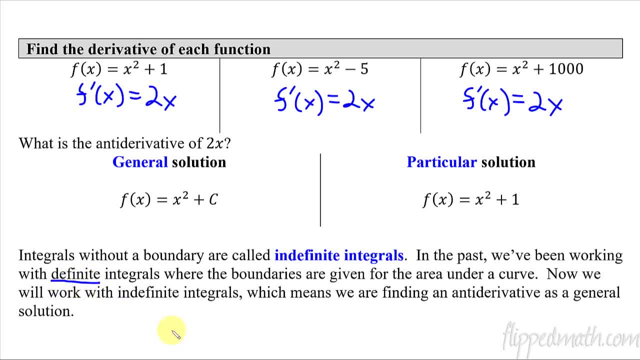 are the ones we've been working with, where we are taking the area under the curve and we go from point a to point b. Those are definite, So today is indefinite, and the solutions to indefinite integrals have this plus c, So they're in the form of a general. 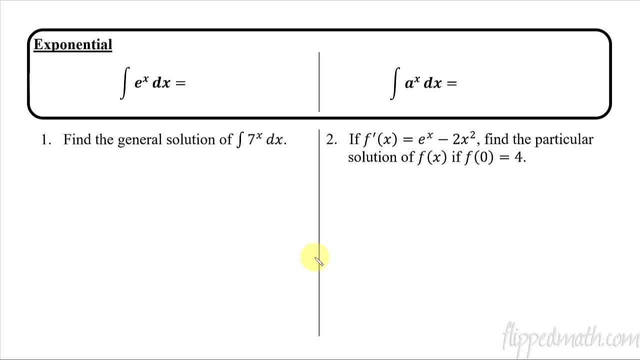 solution. Okay. so let's do some examples Exponential. We're going to start off with this really easy. Whatever, the answer here is: the derivative of it would give us e to the x. That's how you do antiderivatives. If you take its derivative, does it give you what you started? 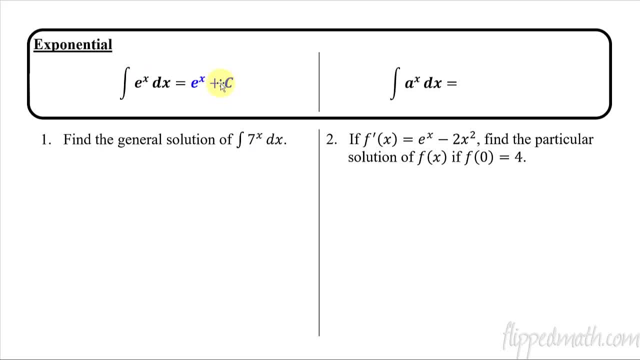 with which is e to the x. So this one's pretty straightforward, because it is just e to the x. Remember, the derivative of e to the x is e to the x, so it's e to the x plus c. That's our general form. This one's a little bit trickier and I 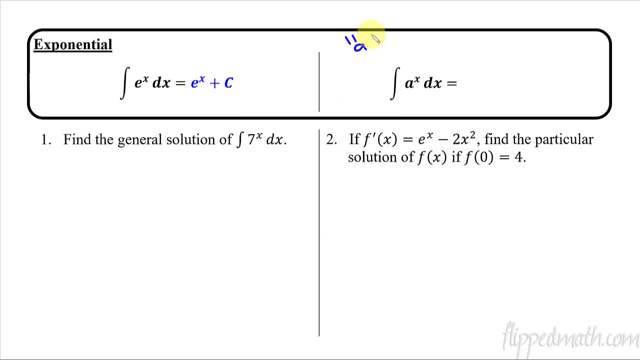 forgot to put something on here. I should have some statement about what a is. A is, let's call it a. a is a number greater than zero. Yeah, we don't want it to be negative for this exponential to work. So we are saying a to the x, its derivative, Now off on the side of your notes. 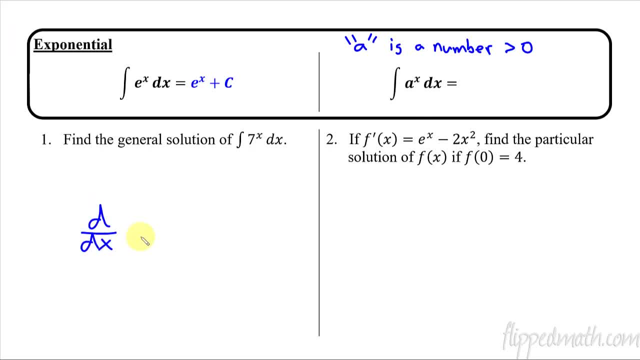 there's something down here, but don't do it down here, Maybe off on the left side. Let's just remind ourselves really quick what is the derivative of a to the x? It is a to the x, and then you remember this times the natural log of a. So if you were working backwards, the 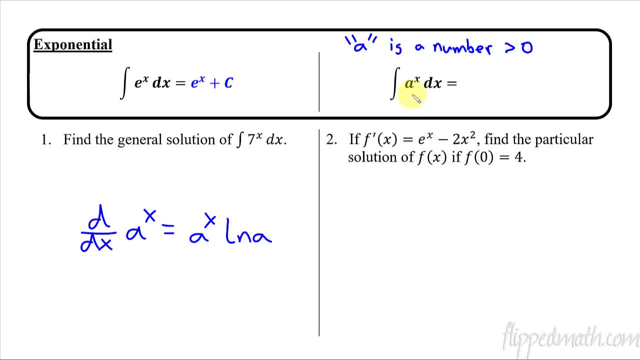 other direction. how can you take the integral of a to the x? Like? what in the world would that give you? So it has something to do with this. So this would be a point in the lesson. if I was teaching you in class, I would make all of my students: hey, see what you can come up with. 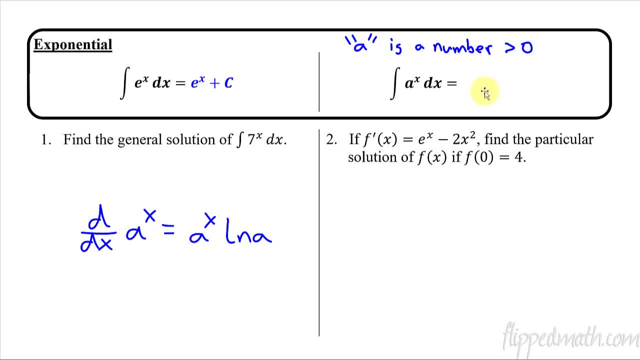 Do you think you've got it? Maybe check with each other. It's a good chance for you to pause right now and just try and see if you can come up with it on your own. So try it first, And then here's the answer. So pause, pause, Here we go, The answer. 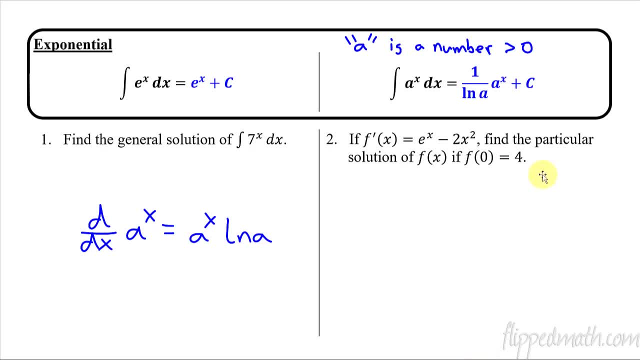 is one over natural log of a times a to the x and then plus c for your general solution. Now, if you look at that part of it right here, this part, if you take its derivative, you would take it: the one over natural log of a is like a coefficient, So you just take the. 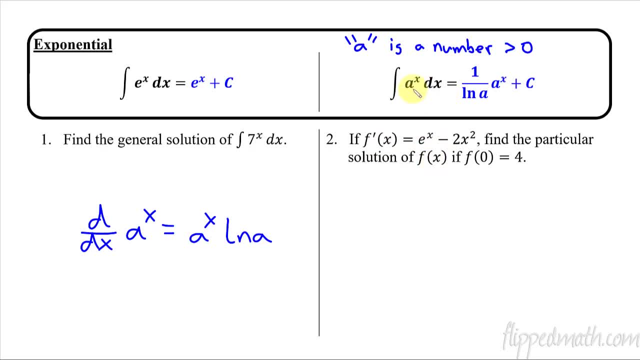 derivative of that. And then you'd see here, the natural log of a's would cancel, And that's how you'd get back to this one. So let's find the general solution of this first one. So we just follow the pattern. 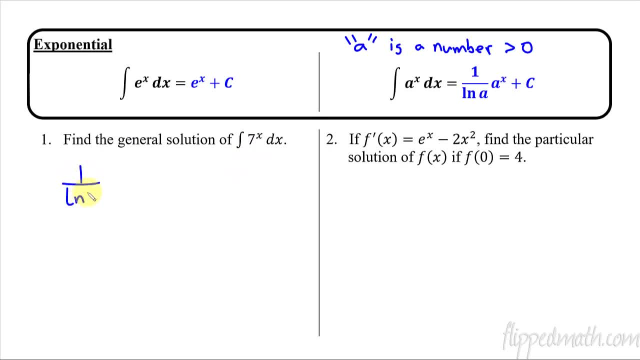 There. the answer to that is going to be one over the natural log of seven. So again, this is antiderivative, not derivative. That's when you have the one over, if it's the antiderivative, and then times seven, raised to the x, And then we have our plus c for the general. 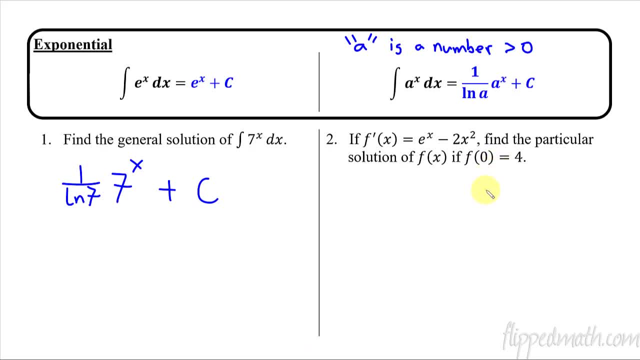 solution. Here we're going to do a particular solution, So this is the first time we've done this. So we take the antiderivative of this, So f of x, and we first write it in the general solution form. So the antiderivative of e to the x is itself e to the x minus. And then here: 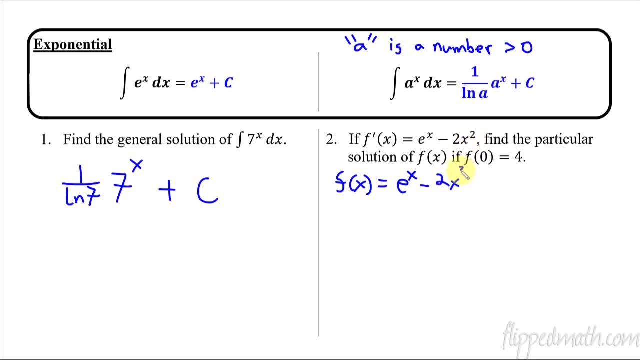 we get two x to the add one. you get three divided by three, And then we have to have our plus c for our general solution. Notice I'm writing small to leave myself some room. You want to do the same, Okay, so. 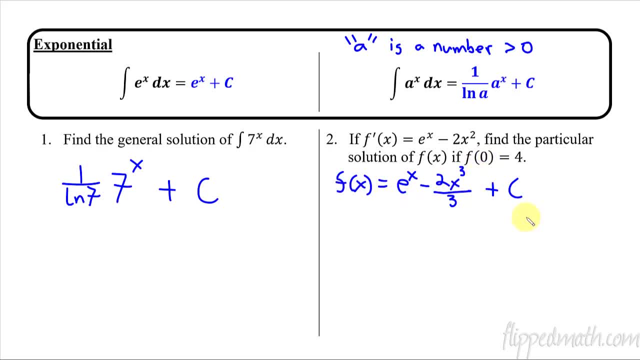 now we take what? instead of a general solution, we want the particular solution that fits this criteria, where x is a zero and y is a four. So y is four and then x is zero minus. that whole thing becomes a zero if x is zero plus c. And now we find the general solution, So we take the antiderivative. 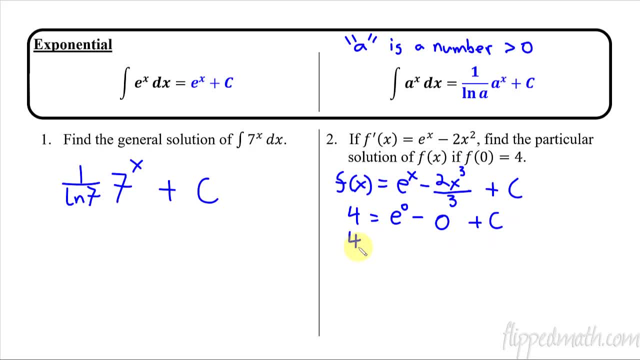 to figure out what c value fits this criteria. So we have four equals one plus c. subtract the one, you get three equals c. So now we can write out the answer. The particular solution is: f of x is going to equal. so it's this line right here: e to the x minus two thirds x cubed. And now instead: 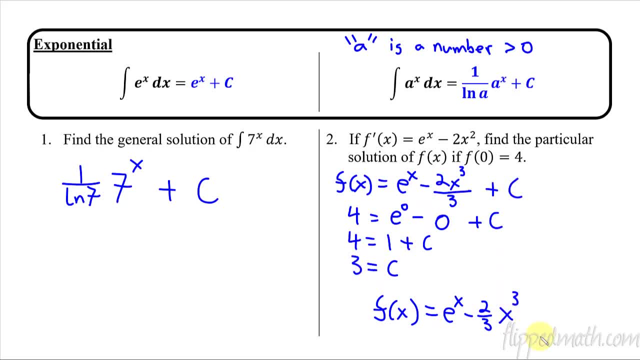 of a plus c. we write what c actually is plus three. So this is our particular solution that fits the criteria. that is the antiderivative of this, And then we take the antiderivative of this and then we figure out exactly which c it is that we're talking about by using the coordinate. 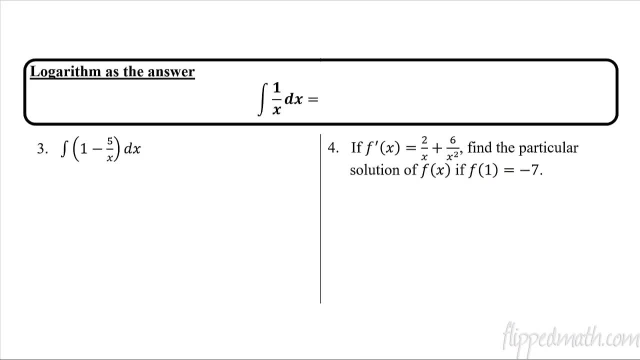 point. plugging in the points. That's how you get the particular solutions to these. Next up, we have logarithms as the answer. So we have here one over x. When you take the integral of one over x, you get the natural log of x. But we have to include this weird absolute value. I will talk. 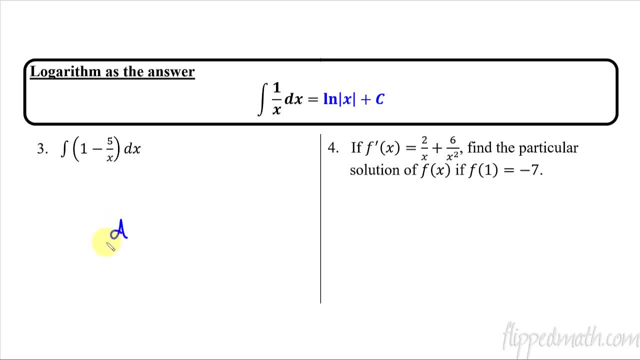 about that in just a minute, But just as a reminder, when you take the derivative of the natural log of x, remember that you get one over x, So it would make sense. if you're doing the antiderivative, don't write this here, by the way, this was just a side note. If you do the antiderivative, 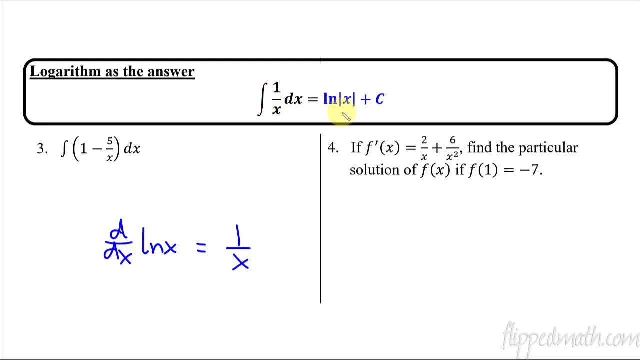 you'd go back to natural log of x. Now the qualifier here is that it must be absolute value around it. Because, whatever your answer is, if you remember the logarithm graph, it does something like this: where you have a vertical asymptote and you aren't going to have x values. 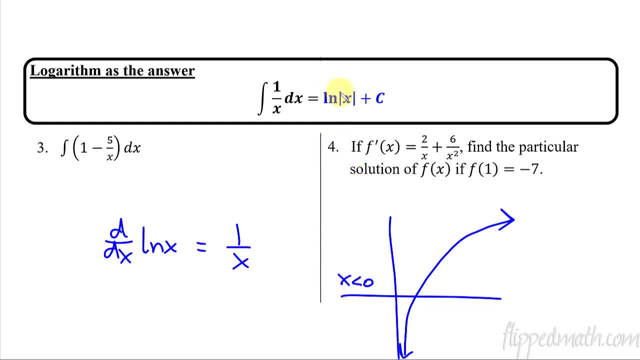 that are less than zero in a logarithm function, And so we have to put these absolute values around that. So, just as a reminder, usually this comes up in a multiple choice type problem And they'll have the absolute values in the multiple choice. So it makes it a little easier And 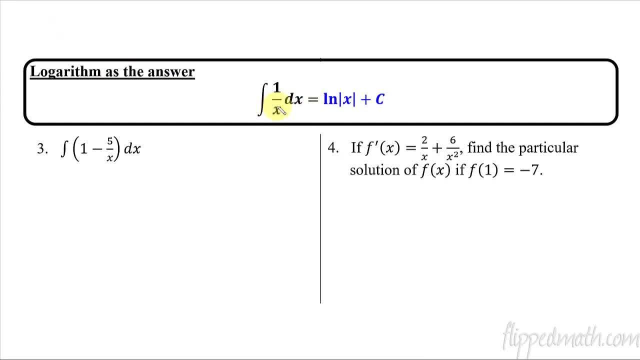 sometimes kids get confused on when to use the logarithm. So let me show you. if you tried the antiderivative power rule, like the inverse of the power rule, and we change this to x to the negative one, and then you were to add one to it, you'd get x to the zero divided by zero. you can't. 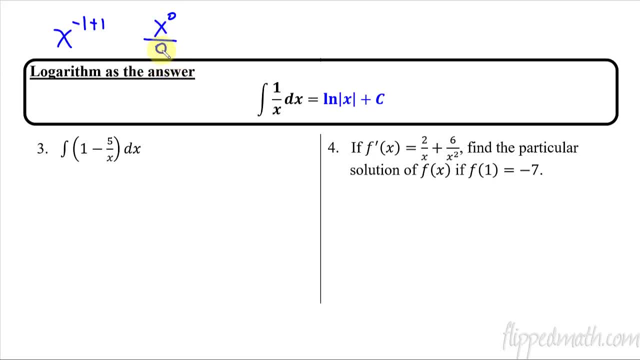 divide by zero. So hopefully, if you were to just try that, you'd see there's a problem there And that would trigger a memory. Oh yeah, that's because this is just becomes the natural log absolute value of x. That's what that one has. 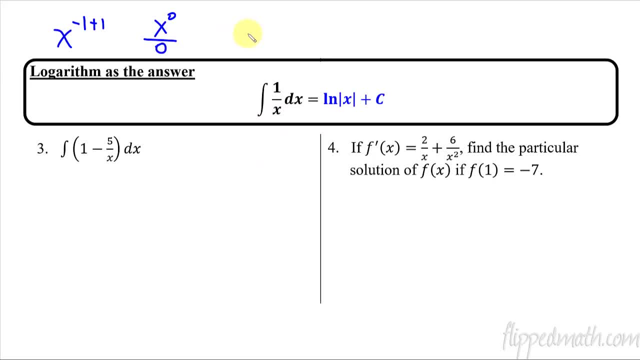 And don't be confused. This is: this is a very common mistake. When kids see this one over x squared, they'll go straight to an answer and think, oh, that's the natural log of x squared plus C. No, it's not. Don't do that. Okay, don't do that. You only have this natural log when it's. 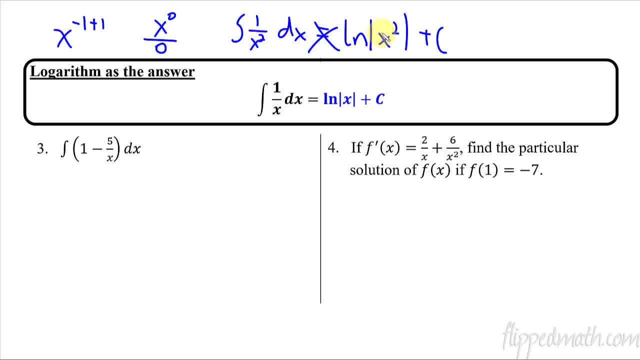 one over x to the first power. If it was one over x to the second power, then you do the normal things that we've been doing before with the this power rule thing. Okay, so let's take this example, which is just x minus, and now that five can just be pulled out, And then it's like it's one over x. 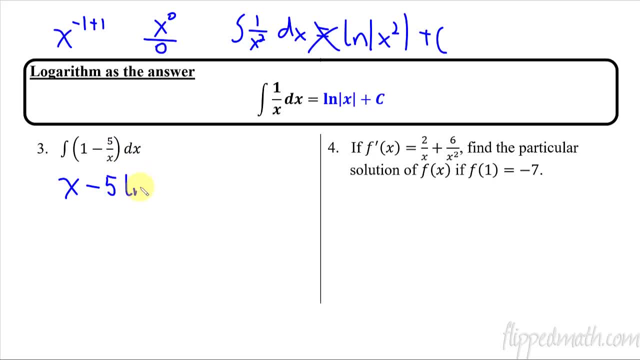 five times one over x, And then the antiderivative one over x is the natural log of x with an absolute value there, And then we add our constant C. Okay, and then that's it. So now let's do one with a particular solution instead of just a general solution. So I'm going to have f of x. 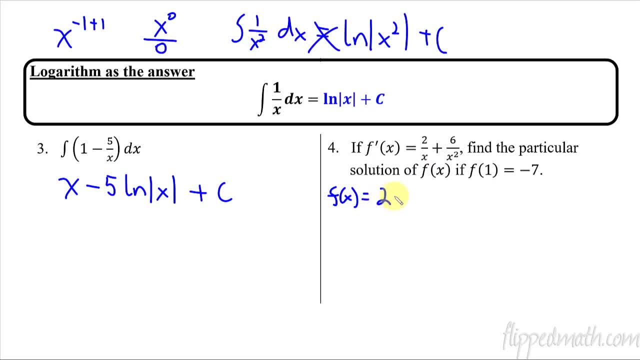 is going to equal. So here I have two natural log: absolute value of x and then plus. now what's going to happen here? let me do some side work up here: six x to the negative two if I add one, so it's going to be x to the negative one, and then I would have to divide by negative. 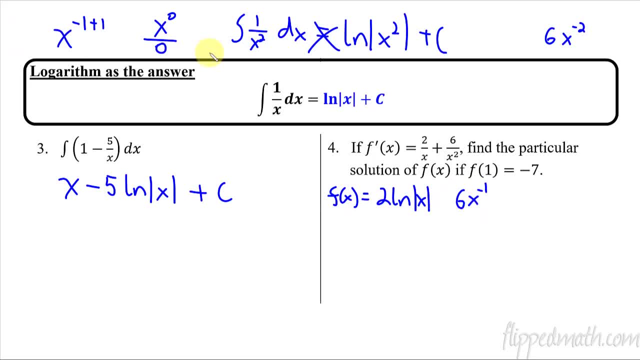 one, Or I could just change this little plus symbol to a minus, And then that'll save me that step. So instead of dividing by negative one, I change the plus to minus and then I add my C. Okay, now we plug in the point one negative seven. So negative seven is my y, And then I'm going to 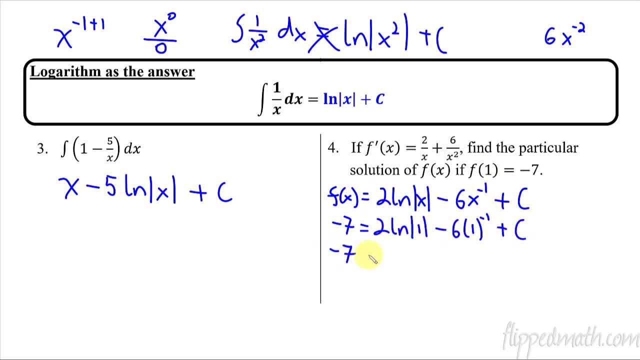 plug in one And then from there it's just simplifying. But you do have to remember the natural log of one is zero, So that whole thing is a zero. And then you're just solving for C from there And you get the C equals negative one. So now we can write what f of x is. 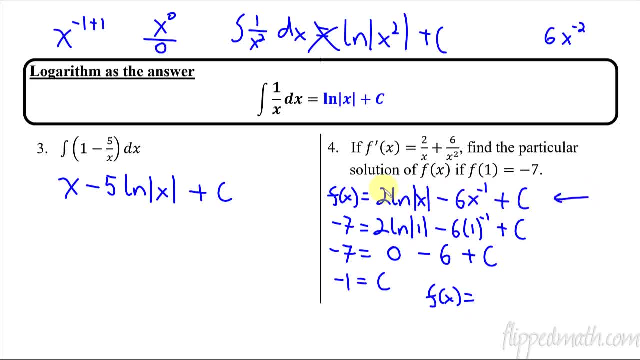 And where do I get that from? It's this line right there. f of x is this, So that we just plug in what the C equals. So it's two natural log absolute value of x. And then this I can simplify to six: 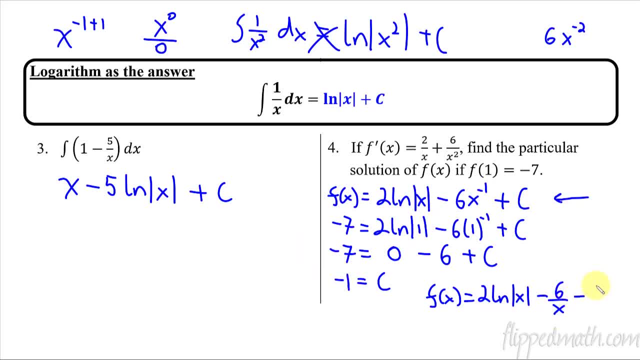 over x, And then the C is a minus one, So I'll say minus one at the end. And there's our particular solution to this derivative. And then I'm going to plug in my y, And then I'm going to plug in my: 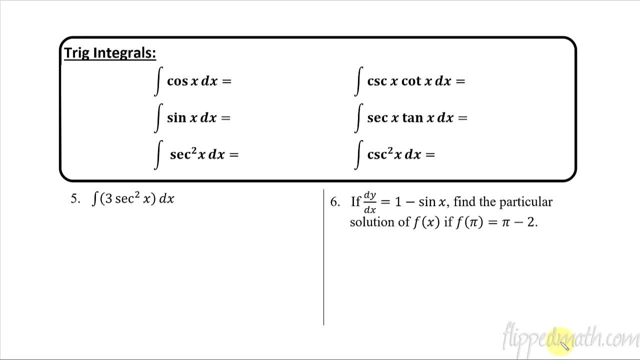 derivative. It's the function that goes through that point. Trig integrals: Now we're again with trig integrals, we're just going backwards from their derivatives. So we already covered these first two in our last lesson. which is sine x, the antiderivative of cosine x is sine x. 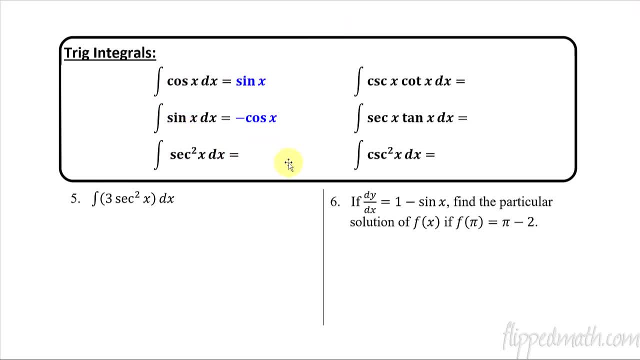 the antiderivative of sine x is negative cosine x. So hopefully you can look at these and kind of remember. okay, what derivative do we take that gives us secant squared? That one's just tangent x. Oh, I forgot something important, Oops, sorry. Plus the constant: 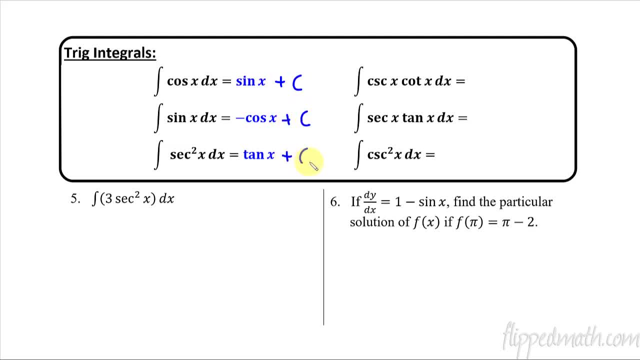 these have got to be general Plus c plus c. I'll get that fixed on this one. So then on these we have these answers: Cosecant cotangent is the derivative answer of negative cosecant x, Secant x. tangent x is the derivative answer of secant x. So therefore you can go the other. 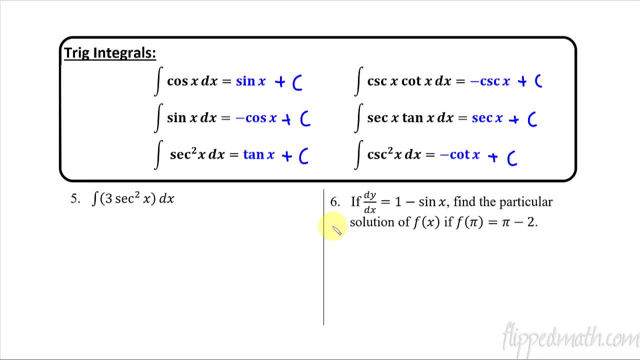 direction for the antiderivative. So if you don't have your trig derivatives memorized, this is hard, You have to have those down by now, And so, again, you want to spend some time memorizing those. If you don't have them yet, I will give you one hint, And that is for this: the signs. 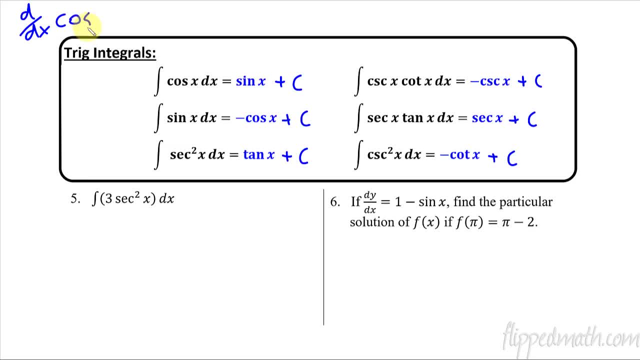 whether it's negative or not. Remember, when we take the derivative of a trig, if it starts with a c, then you have a negative answer, right? If the derivative starts with a c for trig derivatives, then you have a negative answer. It's negative sine x. Well, if it's an integral, then it's if. 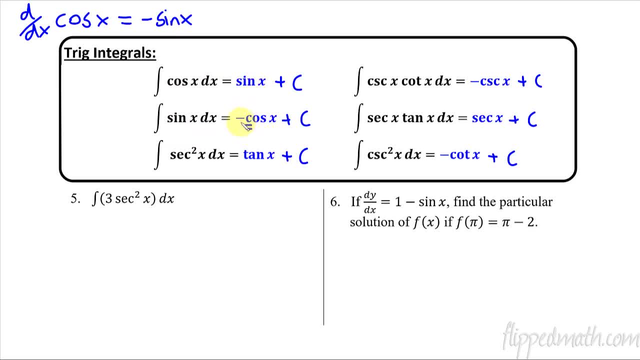 the answer starts with a c. So notice this: If the answer starts with a c, you have a negative answer. If the answer starts with a c, it's negative Answer. starts with a c, then it's negative. That's when they're negative. 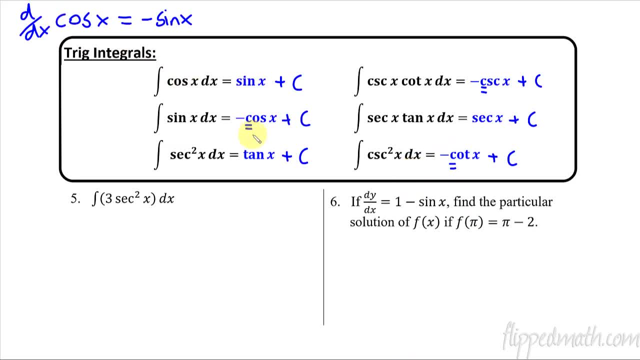 only when the answers are So derivatives. if it's when you start with a, c, integrals. if your answer is a, c, All right, so this one right here: three secant squared. that one's pretty straightforward. Secant squared is just the answer to a derivative. 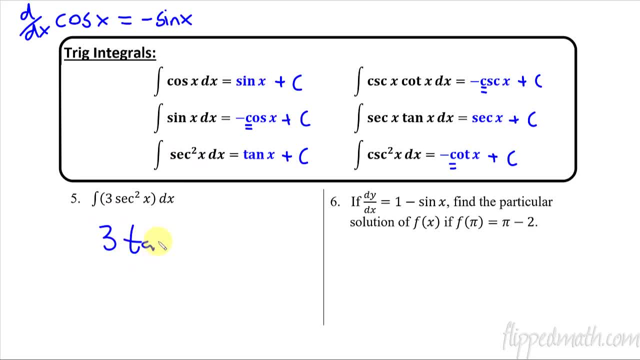 problem of tangent x. So this is three tangent x plus some constant for our general solution, And now we'll do the particular solution. So we're going to say y equals antiderivative, one is x, and then minus the antiderivative sine is cosine. But since the answer starts with a, c, we have to take the opposite. 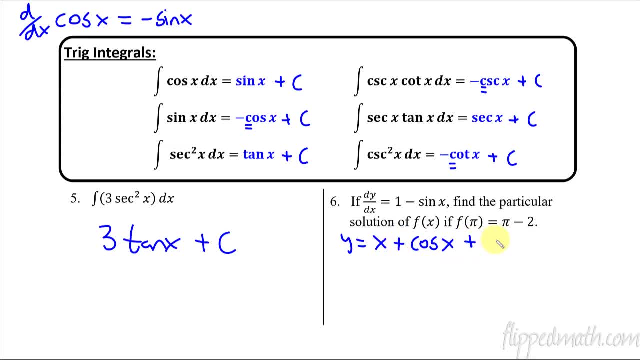 sign. So now we'll make it a plus and then we add a constant. Okay, now I did not leave myself in a lot of room, Sorry about that. Now, this pi minus two, that's the y value. So pi minus two equals. 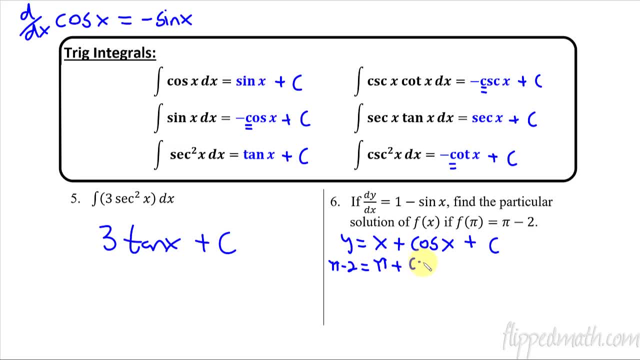 the x is a pi. So we go pi plus cosine of pi plus a constant and then subtract the pi's, we get negative two. the pi's cancel Cosine of pi is negative one plus c. Add the one over here, we get negative one equals c. All right, so now here's our answer. 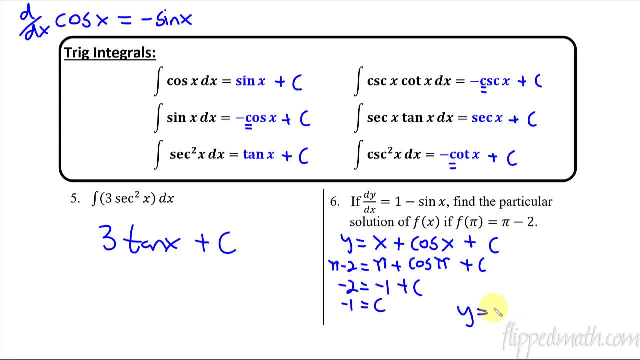 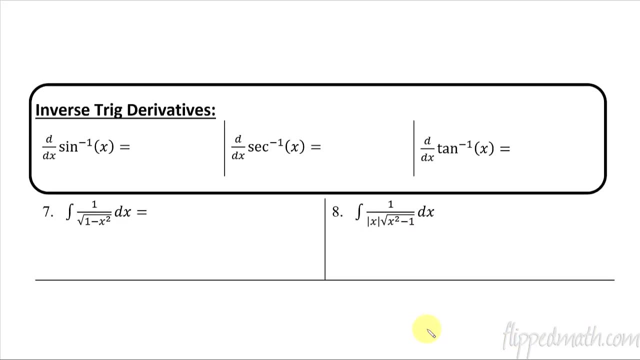 y equals y equals x plus cosine x, and then the plus c in this example is a minus one. So there is our particular solution for this scenario: Antiderivative, and then you use this coordinate point to plug it in and find your c. Inverse trig derivatives are not that hard, if you remember. 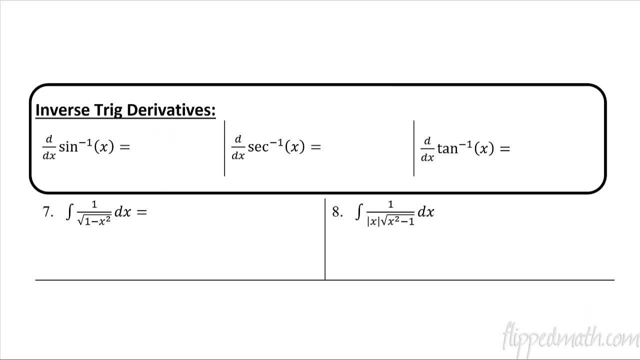 them. If you don't remember them, then yeah, there's no way you're getting these right. So, just as a reminder, I have here the trig derivatives, not antiderivatives, but just the trig derivatives, And that is. 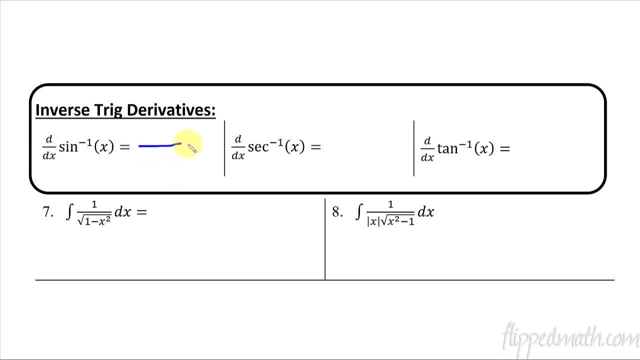 remember that if it starts with an s, so remember this, if it's always going to be one over, and then if it starts with an s, it's the square root and subtraction. So then we have: is it the one in front or the one behind The sine, remember? I like to think of that. 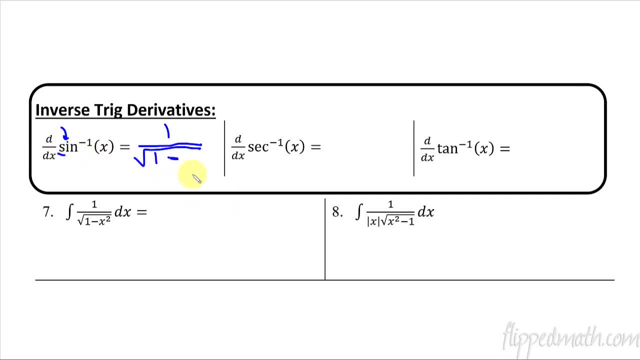 i as like a one to remind me that the one comes first, and then it's x squared, And then the secant. it also starts with an s. So I've got one over a square root symbol again and a subtraction, So it. 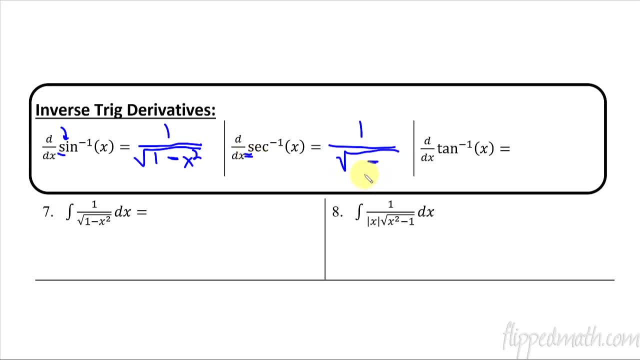 starts with en s. So I've got the square root and subtraction, but the sine is the one with the one first. So this one, the one, comes second. I put an x squared here and then, ah crap, Ah, the c? Crap, I've got absolute value of x as well. I gotta put that little absolute value thing on. 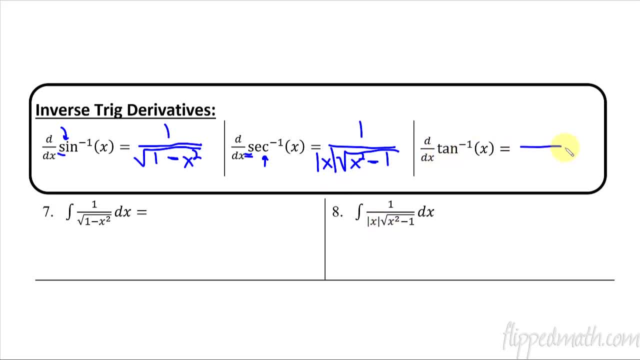 the bottom in the denominator and then tangent does not start with an s, So we just go one over over. so there's no s, it is addition, and there's no square root. so then we're going to have a 1 and an x squared and it can go either way. it can go 1 plus x squared or x squared plus 1. 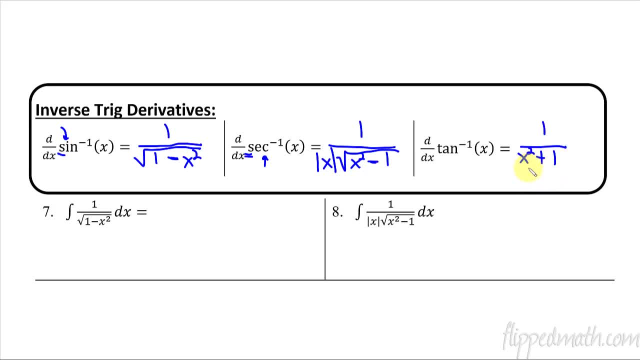 addition is commutative, so the order does not matter. so there's our inverse trig derivatives. so, going backwards, you just have to recognize it. uh, 1 over this thing. what is that? well, the 1 comes first. it's the square root that one's going to be sine inverse of x plus c, or just remember this. 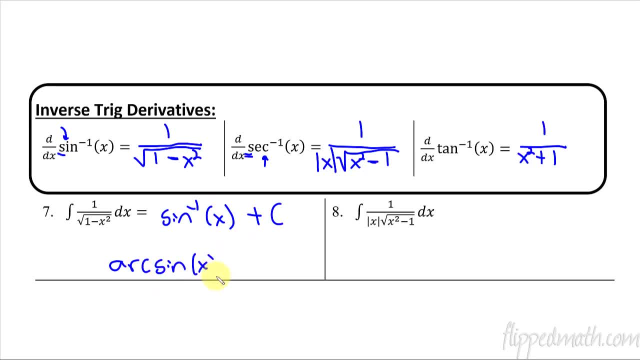 is the same thing. if you said arcsine, so arcsine of x plus c, those mean the same thing. sine inverse or arcsine, so this one, you got the absolute value of x. you got this x squared minus 1. you just try to recognize them. it's easy right now, like i'm showing you this and it's really easy. but if you 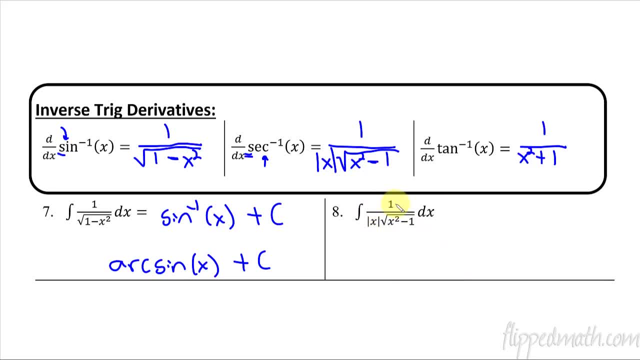 had like two months from now and you're taking a practice exam and you saw this. it's man. what can i remember that like? what is that going on? that's where the hard part comes in. is trying to remember way back here for this lesson. so this one's just secant inverse of x plus c, or we could write that as arcsine. 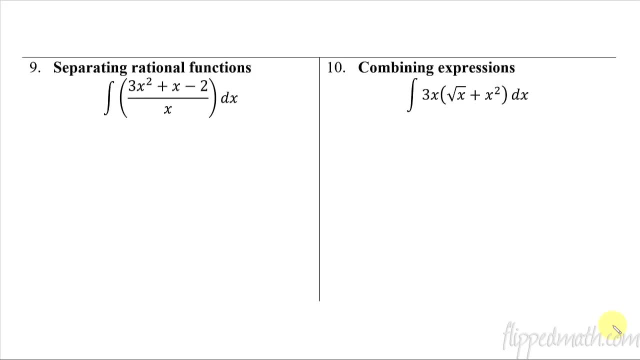 not arcsine, arc secant of x plus c. okay, last two problems and then we're all finished. these two problems are just strategies, algebra strategies, actually how to manipulate these before you take the integral and when you get into higher calculus levels, like a calc 2 and a calc 3, you do a lot of. 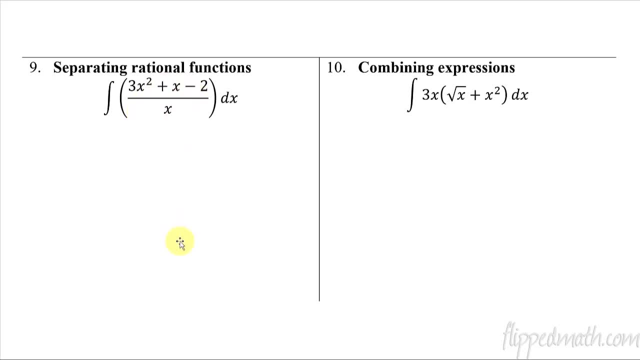 this type of stuff with integrals. you try to manipulate this to make it something you can work with in an easier fashion. so this first one, you- uh, you- separate these rational functions. each of these terms can be divided by x separately, so i'm going to write this as the integral of. 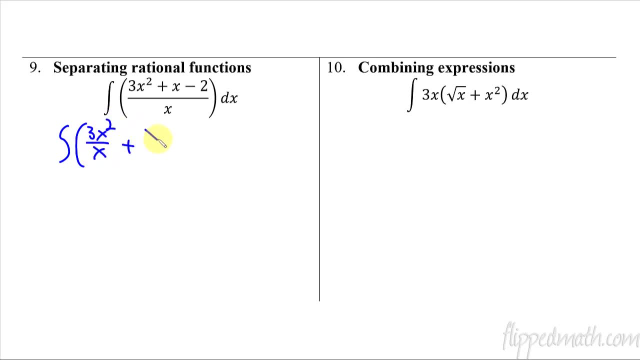 3x squared over x plus x over x, minus 2 over x. so if i can think of it this way and then simplify it, i end up with 3x plus 1, and then this one doesn't simplify, so it's just minus 2 over x. and now that 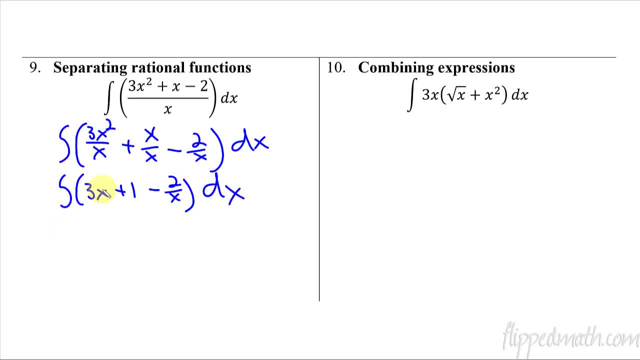 is a ton easier to work with for an integral. so the the antiderivative of this is just going to be 3x squared over 2 add 1 divided by the same number, plus the antiderivative 1 is X. and here's where we have a logarithm, because it's X.